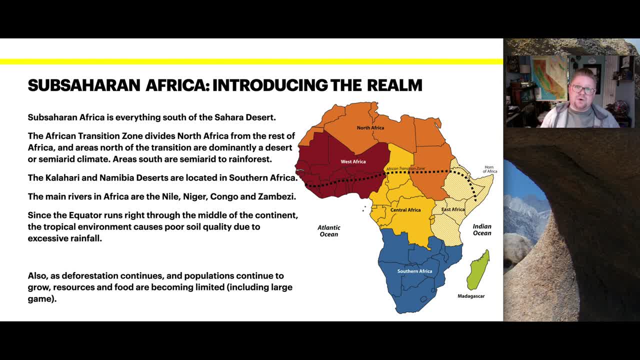 Also, as deforestation continues and populations continue to grow, resources and food are becoming limited, including large game. They're finding that a lot of the large game in Africa is being hunted for food. So the map to the right will introduce the realms that will be discussed today. 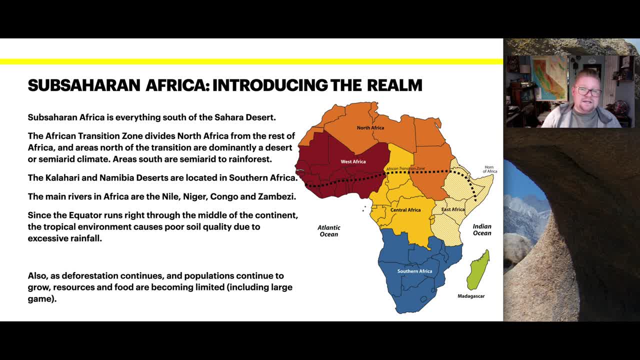 We'll be discussing part of West Africa, Central, Southern and East Africa, So the map to the right will introduce the realms that will be discussed today. We'll be discussing part of West Africa, Central, Southern and East Africa, So the map to the right will introduce the realms that will be discussed today. 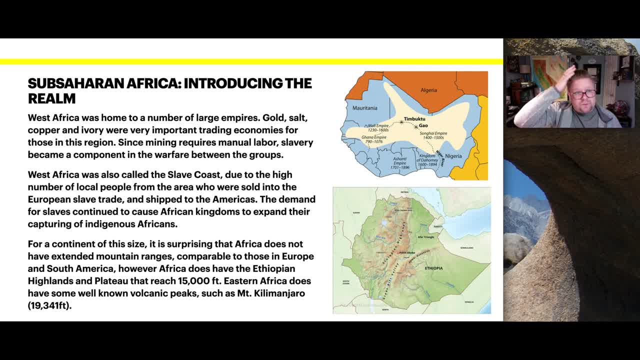 We'll be discussing part of West Africa, Central, Southern and East Africa, So the map to the right will introduce the realms that will be discussed today. We'll be discussing part of West Africa, Central, Southern and East Africa, So the map to the right will introduce the realms that will be discussed today. 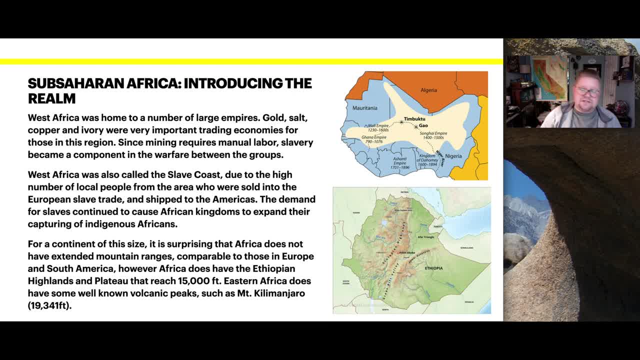 We'll be discussing part of West Africa, Central, Southern and East Africa, So the map to the right will introduce the realms that will be discussed today. We'll be discussing part of West Africa, Central, Southern and East Africa, So the map to the right will introduce the realms that will be discussed today. 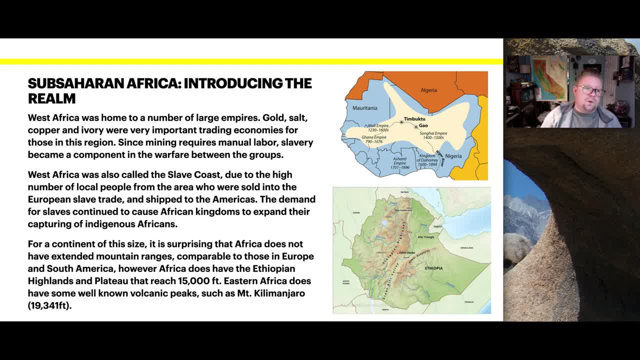 We'll be discussing part of West Africa, Central, Southern and East Africa, So the map to the right will introduce the realms that will be discussed today. We'll be discussing part of West Africa, Central, Southern and East Africa, So the map to the right will introduce the realms that will be discussed today. 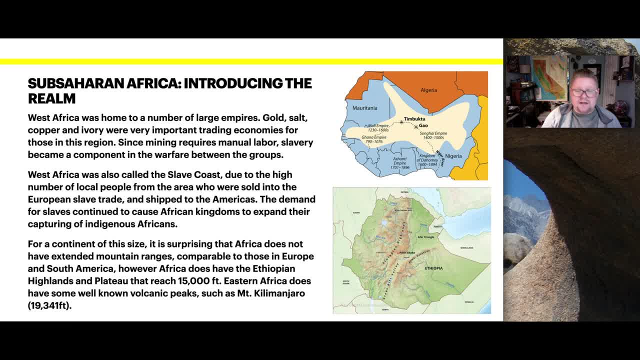 We'll be discussing part of West Africa, Central, Southern and East Africa, So the map to the right will introduce the realms that will be discussed today. We'll be discussing part of West Africa, Central, Southern and East Africa, So the map to the right will introduce the realms that will be discussed today. 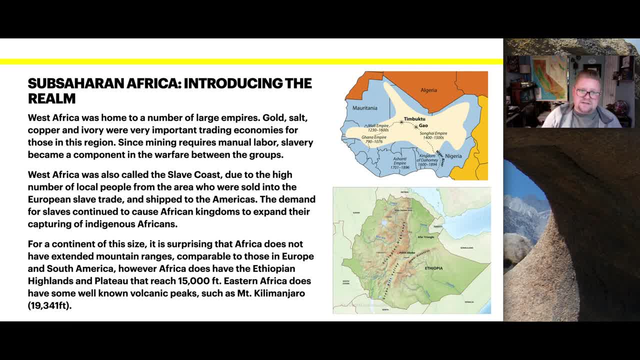 We'll be discussing part of West Africa, Central, Southern and East Africa, So the map to the right will introduce the realms that will be discussed today. We'll be discussing part of West Africa, Central, Southern and East Africa, So the map to the right will introduce the realms that will be discussed today. 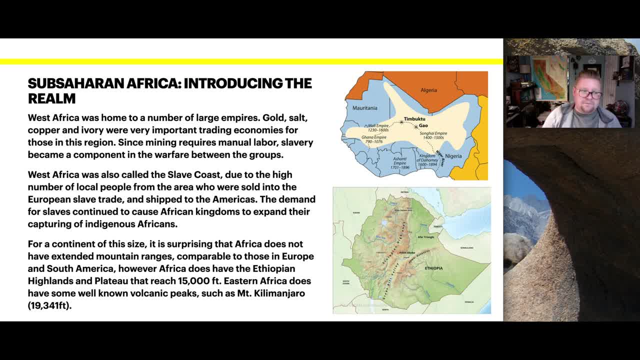 We'll be discussing part of West Africa, Central, Southern and East Africa, So the map to the right will introduce the realms that will be discussed today. We'll be discussing part of West Africa, Central, Southern and East Africa, So the map to the right will introduce the realms that will be discussed today. 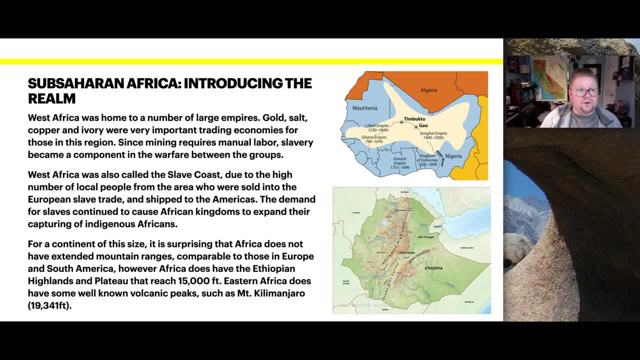 We'll be discussing part of West Africa, Central, Southern and East Africa, So the map to the right will introduce the realms that will be discussed today. We'll be discussing part of West Africa, Central, Southern and East Africa, So the map to the right will introduce the realms that will be discussed today. 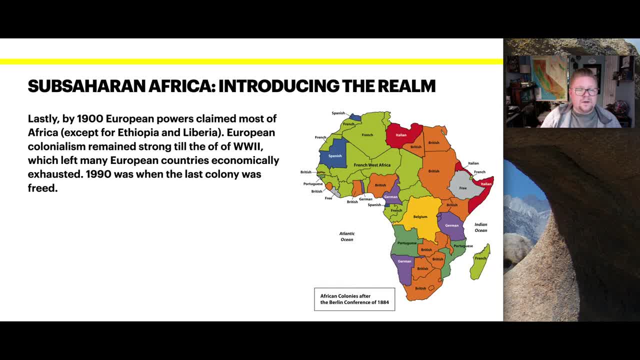 We'll be discussing part of West Africa, Central, Southern and East Africa, So the map to the right will introduce the realms that will be discussed today. We'll be discussing part of West Africa, Central, Southern and East Africa, So the map to the right will introduce the realms that will be discussed today. 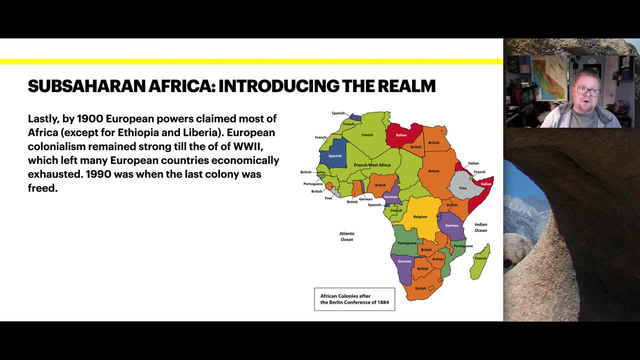 We'll be discussing part of West Africa, Central, Southern and East Africa, So the map to the right will introduce the realms that will be discussed today. We'll be discussing part of West Africa, Central, Southern and East Africa, So the map to the right will introduce the realms that will be discussed today. 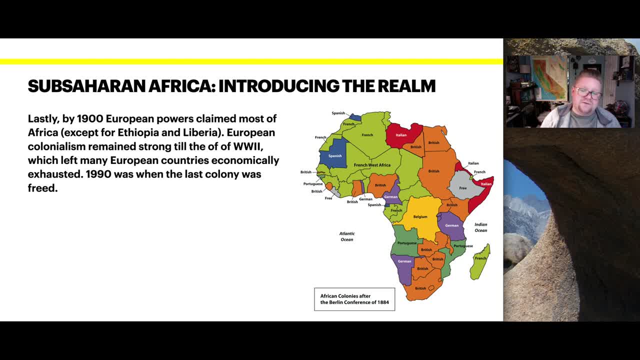 We'll be discussing part of West Africa, Central, Southern and East Africa, So the map to the right will introduce the realms that will be discussed today. We'll be discussing part of West Africa, Central, Southern and East Africa, So the map to the right will introduce the realms that will be discussed today. 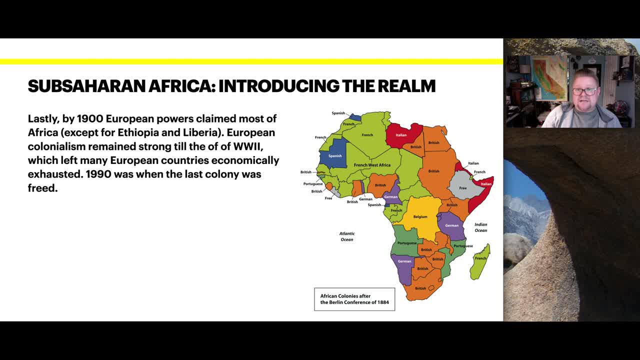 We'll be discussing part of West Africa, Central, Southern and East Africa, So the map to the right will introduce the realms that will be discussed today. We'll be discussing part of West Africa, Central, Southern and East Africa, So the map to the right will introduce the realms that will be discussed today. 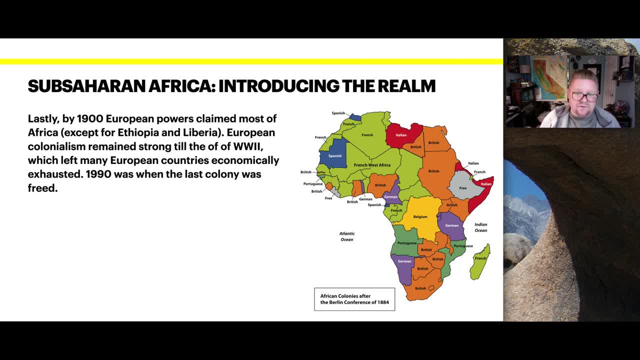 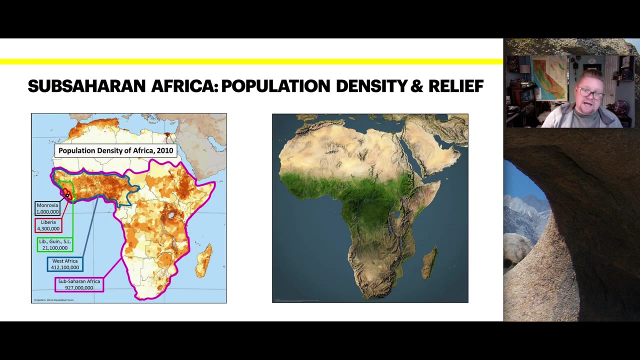 We'll be discussing part of West Africa, Central, Southern and East Africa. So the map to the right will introduce the realms that will be discussed today. We'll be discussing part of West Africa, Central, Southern and East Africa. Let us also introduce the Population Density and Relief Map. 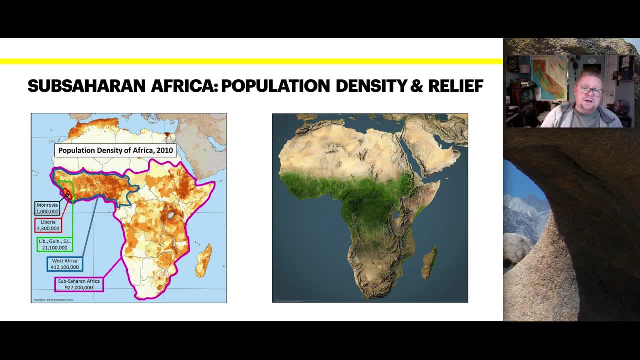 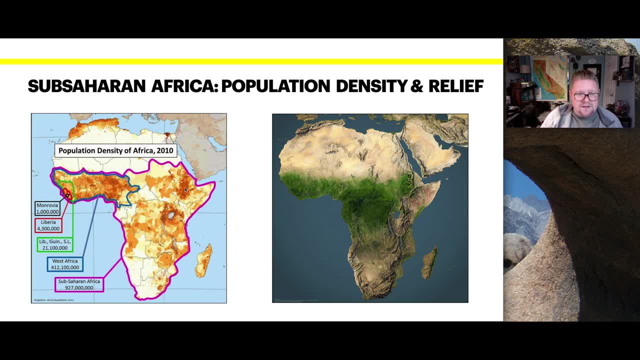 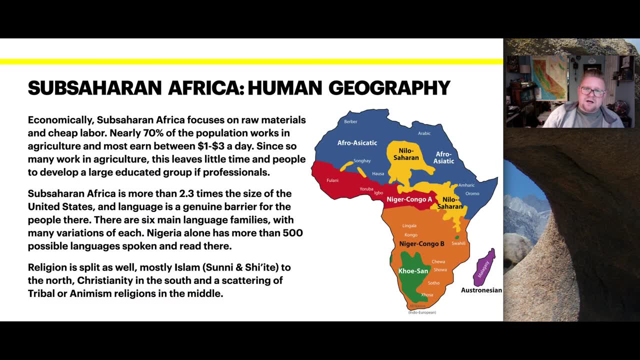 And also we can see that there's a correlation, as we'll talk about in a little bit in eastern Africa. Now let's talk a little bit about the human geography of Sub-Saharan Africa Now. economically, Sub-Saharan Africa focuses on raw materials and very cheap labor. 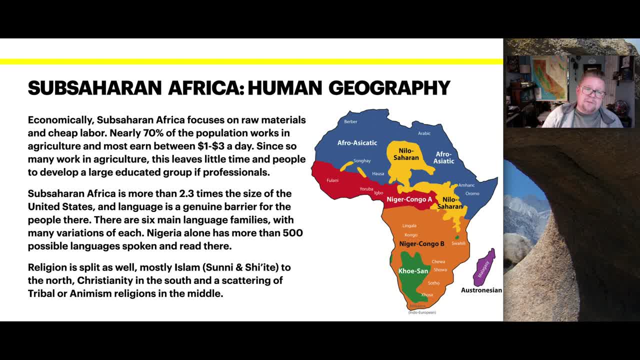 Nearly 70% of the population works in agriculture and most earn between one and three dollars a day, American dollars that is. Since so many work in agriculture, this leaves very little time and people to develop a large educated group of professionals. 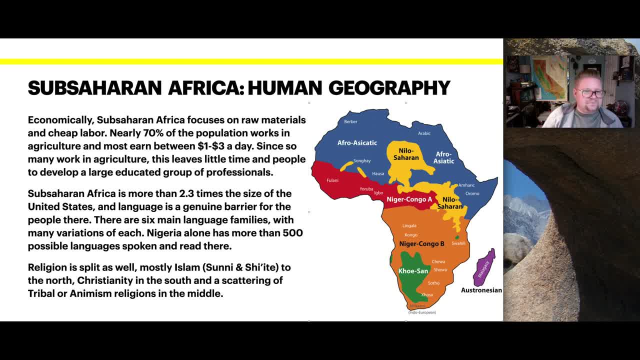 Sub-Saharan Africa is more than 2.3 times the size of the United States, and language is a genuine barrier for the people that live there. There are six main language families with many variations of each. Nigeria alone has more than 500 different languages spoken and read there. 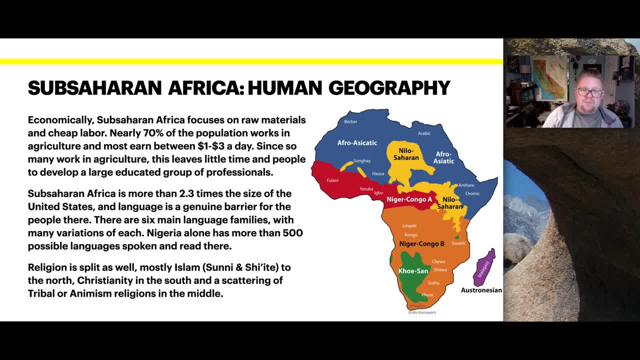 and red. there. Religion is split as well, mostly Islam, which is Sunni and Shiite, and those are to the north, as well as Christianity to the south and a scattering of tribal and animism religions in the middle. So this diagram here on the right of Africa is just really distinguishing the 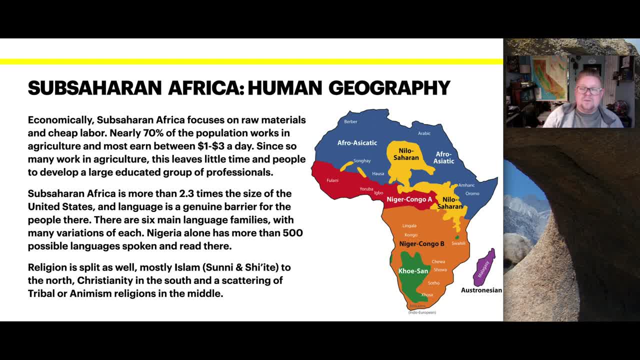 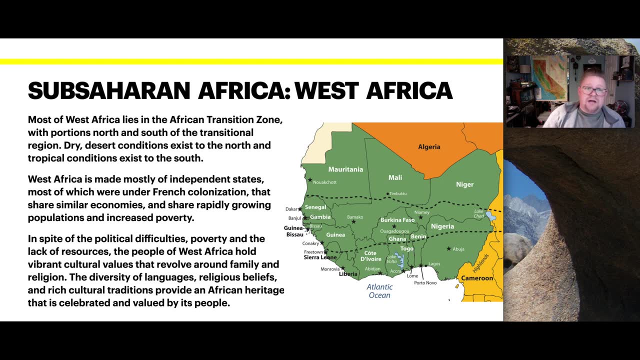 different language groups that are identified, But again, each language group has its own variation and style that can be very, very different. So let's introduce West Africa. Most of West Africa lies in the African transition zone, with portions north and south of the transitional region Dry. 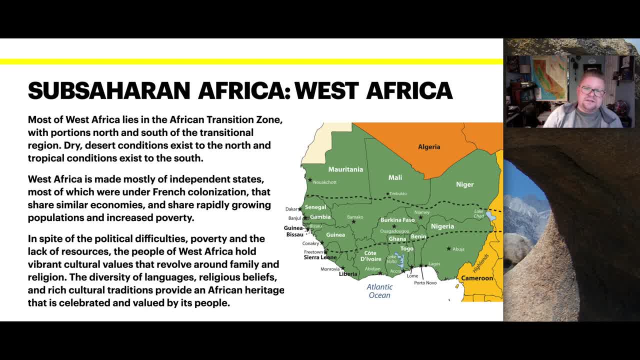 desert conditions exist to the north and tropical conditions exist to the south. West Africa is made mostly of independent states which were under French colonization, most of, at least, That share very similar economies and share rapidly growing populations and also increased poverty. In spite of the political difficulties, poverty and lack of natural resources for 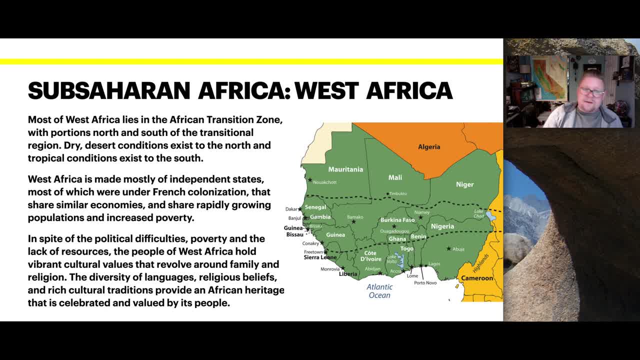 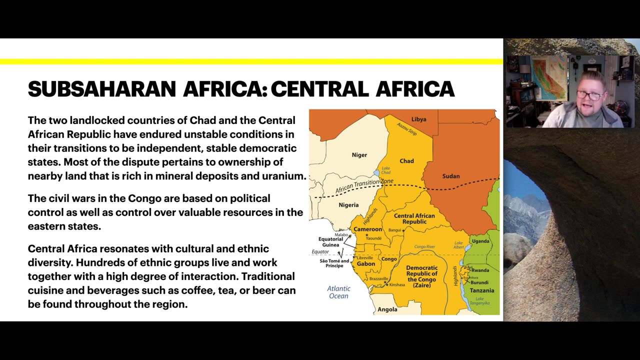 themselves. the people of West Africa hold vibrant cultural values and revolve around family and religion. The diversity of languages, religious beliefs and rich cultural traditions provide an African heritage that is celebrated and valued by its people. Now, looking at Central Africa, The two landlocked countries of Chad and the Central African 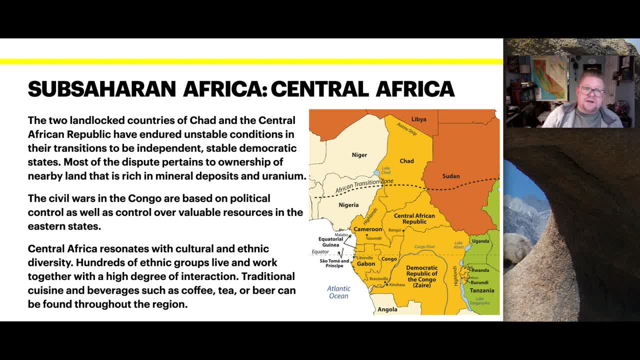 Republic have endured unstable conditions in their transition to be independent, stable, democratic states. Most of the dispute pertains to the ownership of nearby land that is rich in mineral deposits and uranium. The civil wars in the Congo are traditionally based on political control, as well as control over valuable resources in those eastern states. Central Africa resonates with 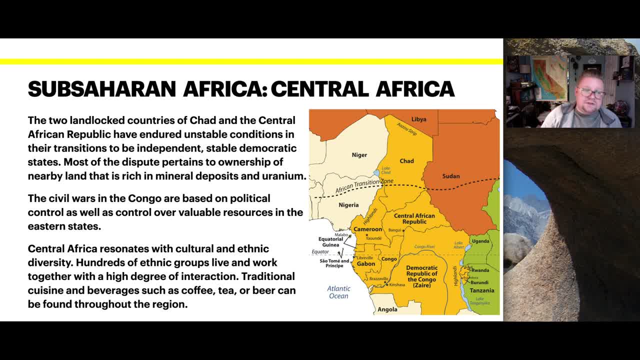 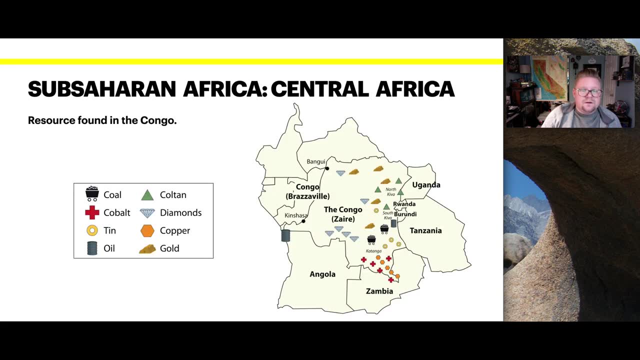 cultural and ethnic diversity. Hundreds of ethnic groups live and work together with a high degree of interaction. Traditional cuisine and beverages such as coffee, tea or beer can be found throughout this region. I also wanted to include this image resources that are found in the Congo. So, as we 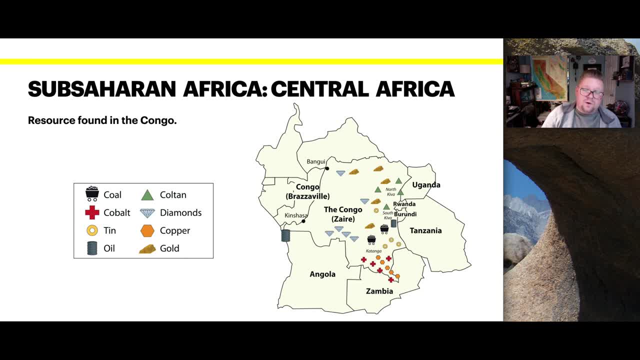 move forward. this is really the driving part of much of the civil wars and really that stress within this region because, as we can see, there's coal, cobalt, tin oil, coltan, diamonds, copper and gold. You probably have heard of all of those, except for coltan. Coltan is used in electricity as high heat. 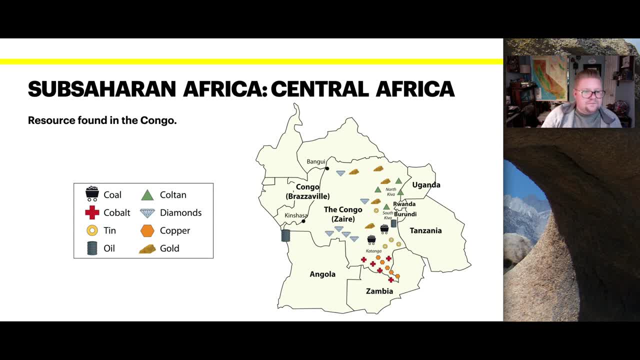 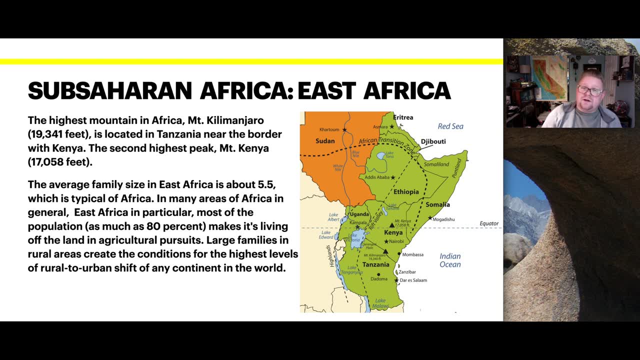 and energy tolerance. So let's look at East Africa. These are the highest mountains in Africa, including Mount Kilimanjaro, which is about 19,341 feet. It's located in Tanzania, near the border of Kenya. The second highest peak in Africa is Mount Kenya at 17,058 feet. 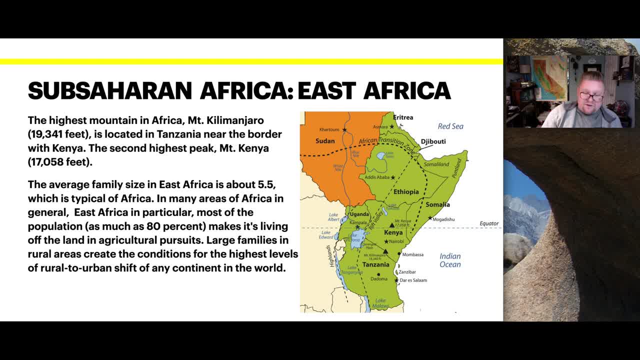 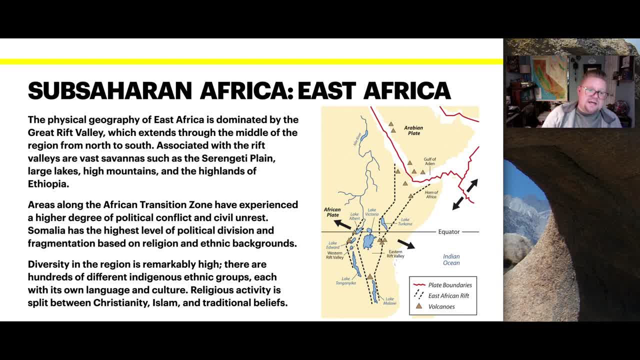 In many areas of Africa, in particular East Africa, is African American. In many areas of Africa, in particular East Africa, is African American. In many areas of Africa, in particular East Africa, is African American, indigenous ethnic groups, each with its own language and culture, religious. 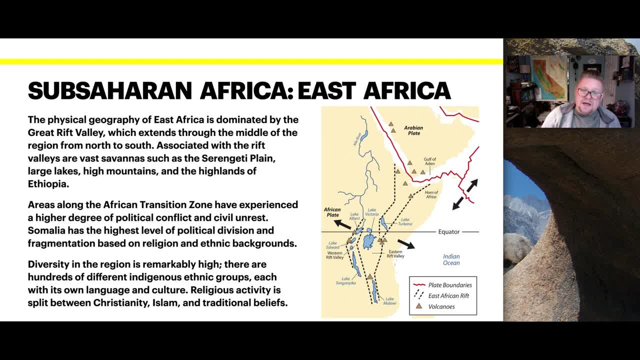 activity is split between Christianity, Islam and traditional beliefs. another thing that I wanted to point out, as we mentioned here, you know this map of East Africa. notice the red line that does represent plate boundaries, so we can see that there is active tectonics, which then leads into the reason and the 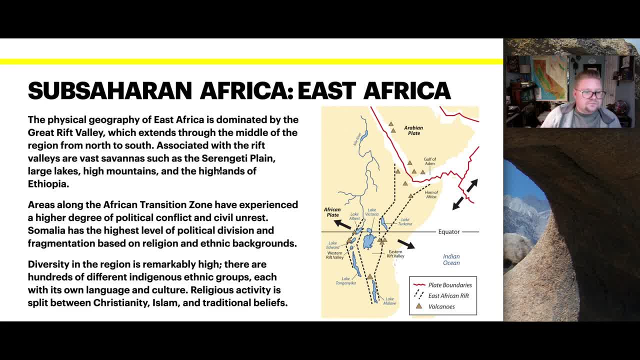 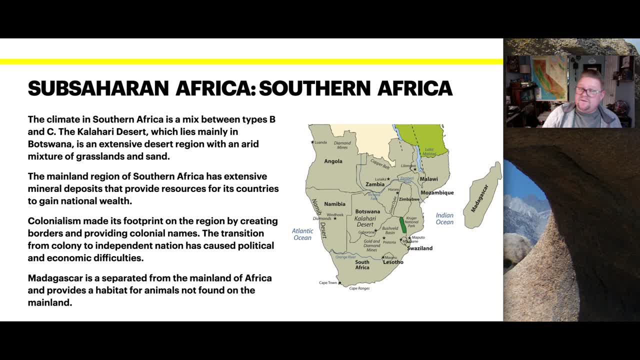 development of that transition zone. so let's talk about southern Africa now. the climate in southern Africa is definitely mixed between B and C types of climates. the Kalahari Desert, which lies mainly in Botswana, is an extensive desert region with an arid mixture of grasslands and sand. the mainland region of south of 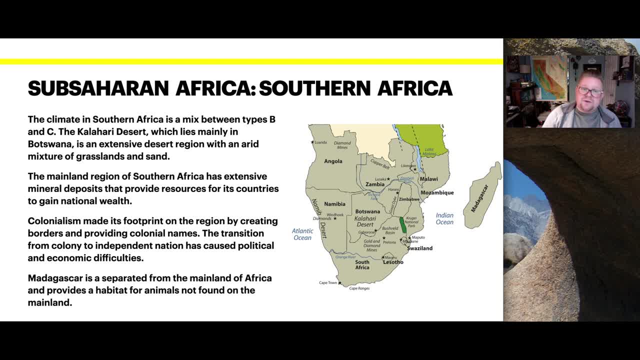 southern Africa has extensive mineral deposits that provide resources for its countries to gain national wealth. colonialism made its footprint on the region by creating borders and providing colonial style names. the transition from colonial to independent nation has caused political and economic difficulties. we also include Madagascar, and southern Africa is separated from the mainland of Africa and provides a 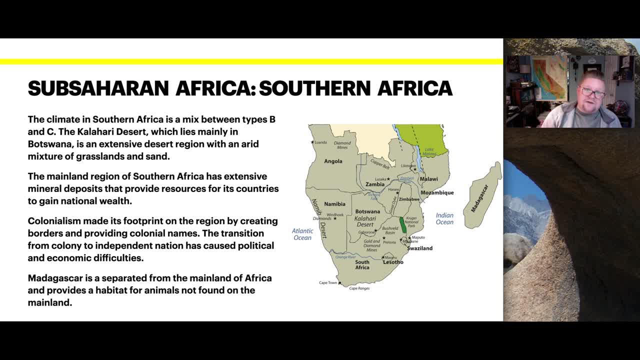 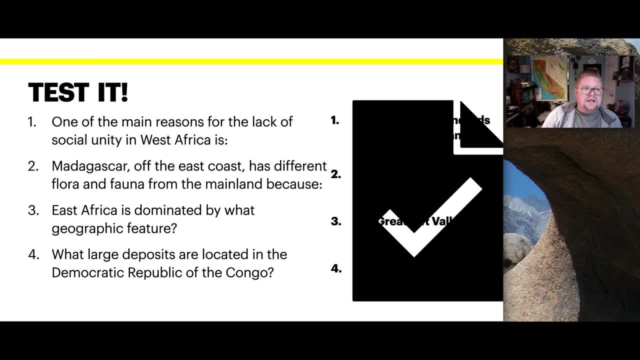 habitat for animals and plants not found on the mainland itself. so so let's test it. I've provided four sample questions here and we'll discuss the answers. the first question is: one of the main reasons for the lack of social unity in West Africa is. the second question: is Madagascar off the East? 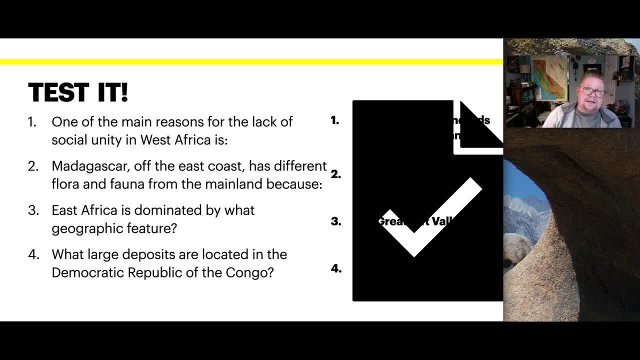 Coast has different flora and fauna from the mainland. because question three: East Africa is dominated by what geographic feature? and question four: what large geographic feature is dominated by what geographic feature? and question four: what large deposits are located in the Democratic Republic of the Congo? don't forget to 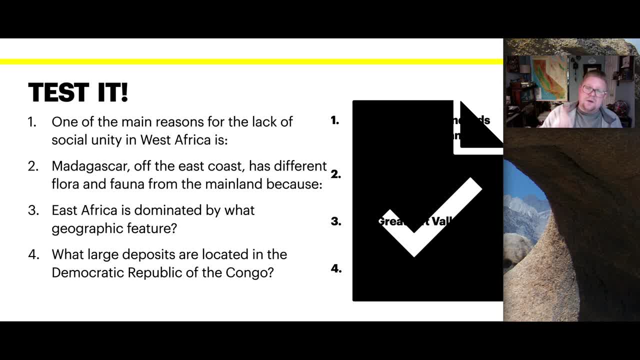 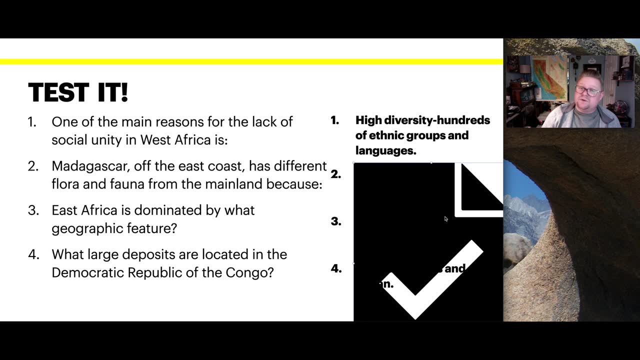 like, subscribe if you haven't done so, and comment with your answers below. so let's talk about the answers. real quick. question one: one of the main reasons for the lack of social unity in West Africa is the high diversity. there's hundreds of ethnic groups and languages and it can be quite challenging for people to 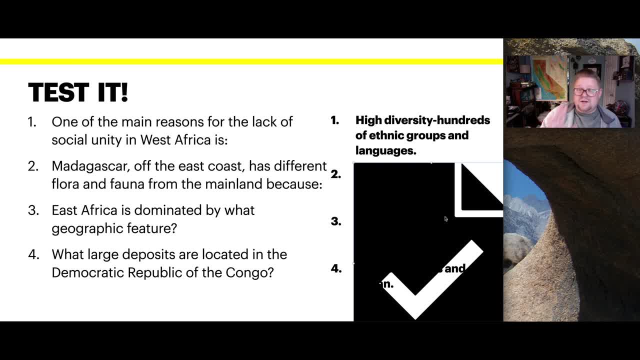 communicate, and that's not just in normal conversation, that's even politically. Madagascar is the third most populous country in the world, with about 75 percent of its population, and it is the first most populated country in the world, with around 100 million people living in it. in the world. 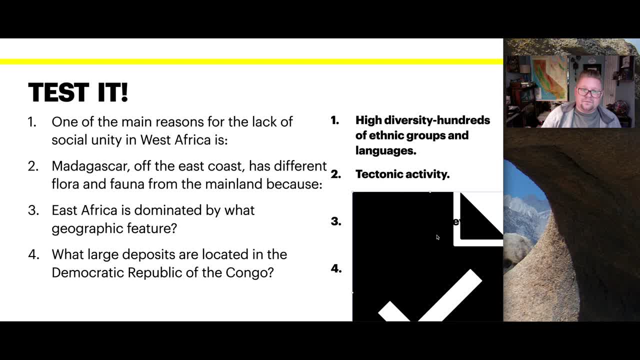 it is the third most populated country in the world, with about 150 million people living in it, so it's not just the only children and youth that are living in West Africa. this is an important point to be aware of, because you know there are a lot of 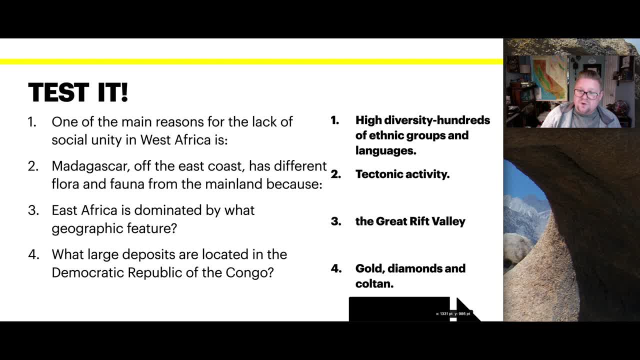 different places in the world, and that's why we want to study in depth and we want to be able to answer as many of your questions as we can, because we want to. was helpful. don't forget to hang around and check out the rest of videos and we'll talk soon.